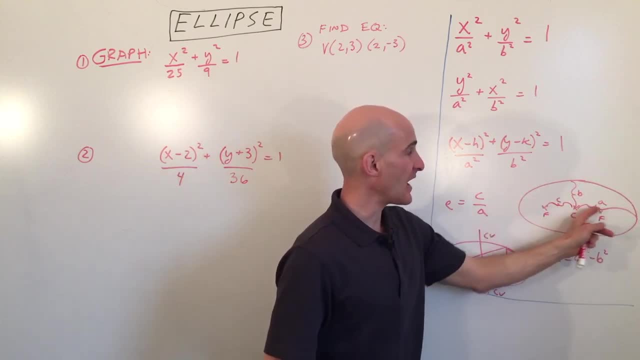 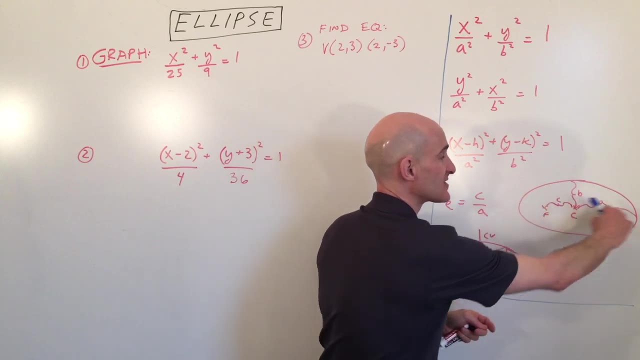 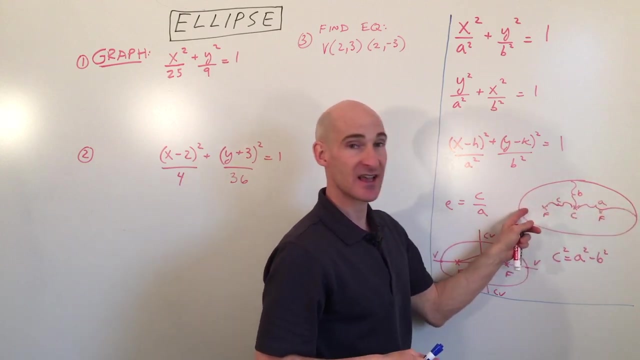 to the vertices: okay, That's the a distance. The distance from the center to the co-vertices: okay, That's where it's narrower. This is the minor axis, This is the major axis. The major axis is the longer axis. So the distance to the major vertices, or just the vertices, that distance. 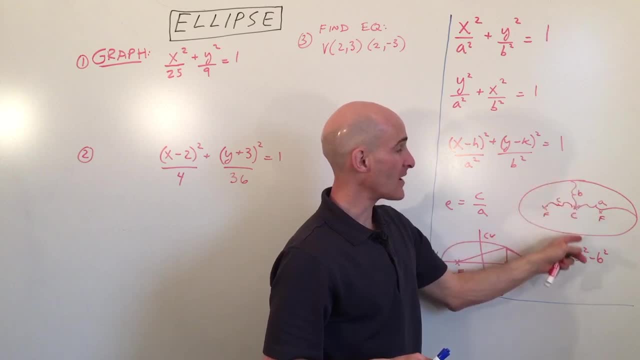 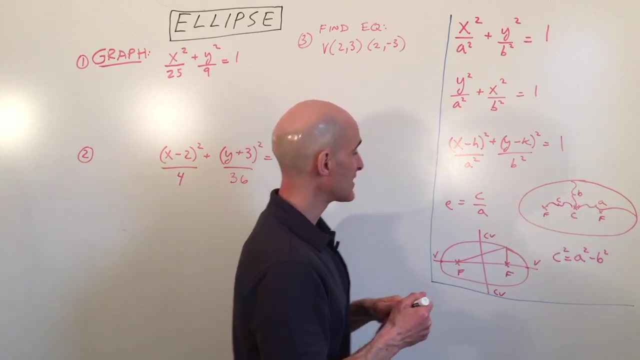 is a: from the center, From the center to the minor vertices or co-vertices along this minor or narrower axis, that distance is b, And then the distance from the center to the foci: okay, these two focal points, that distance is c. Okay, so, basically, what an ellipse is? it's like this, It's: 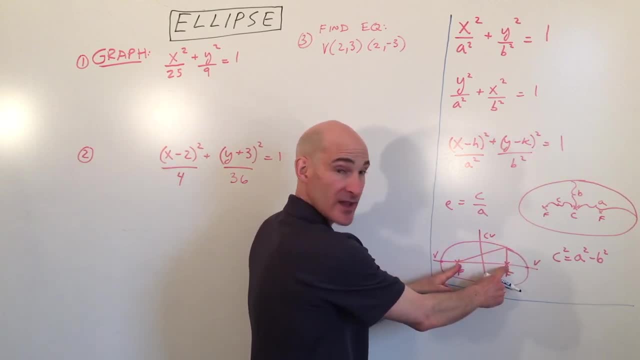 like if you have a string and you hold down the two ends of the string like this: okay, so there's your string and you put your pencil right in there and you pull that string. okay, it doesn't stretch, but the string will gradually get a little bit longer here, but a little bit. 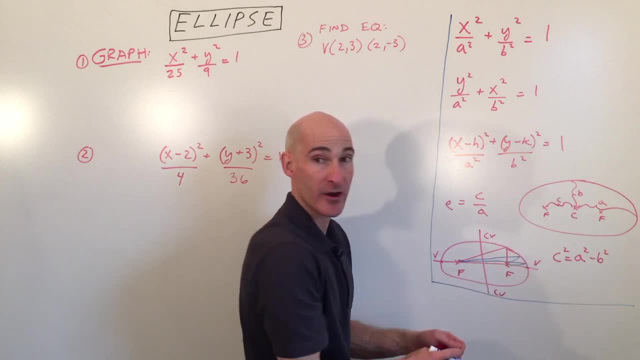 shorter here and then so on. It's going to get a little bit longer here, shorter there. If you take this piece right here- that kind of overlapped- and you cut it and you put it over here, the length of that string will be the length of the major axis. That's called the focal distance, okay, or the? 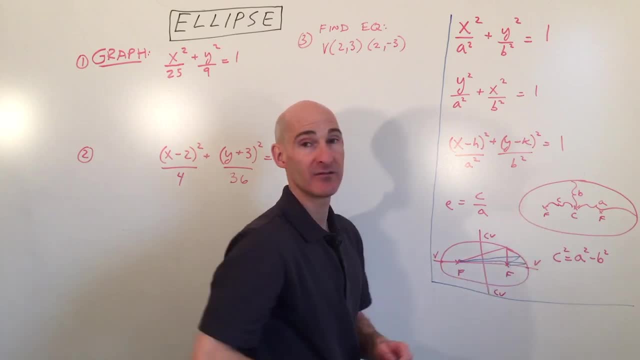 focal length and that's going to be 2a, okay, which is the length of the major axis. Okay. so the a, okay, if it's underneath the y, meaning the larger quantities underneath the y, what that tells you. it's going to be more elongated, okay, or stretched in the y direction, the ellipse, If. 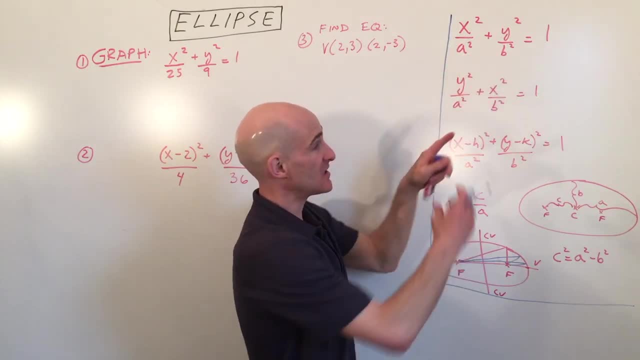 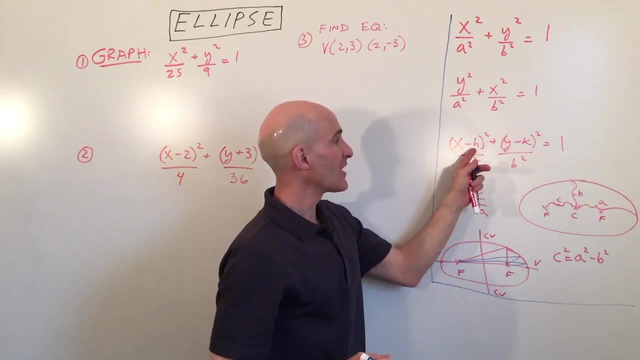 the number underneath the x is larger between the two of these, it's going to be more elongated in the x-axis direction, like the horizontal direction. Okay now, just like we work with parabolas, with shifting them, you can shift these ellipses as well using this h and k. So h and k. 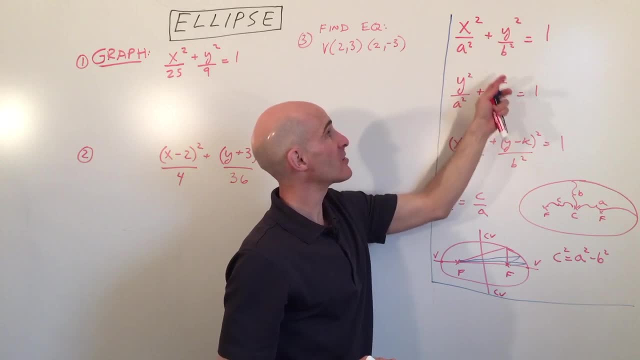 is the center of the ellipse. So if there's not an h and k, like here, it's going to be the center of the ellipse, It's going to be at the origin, okay. So let's get into some problems and I'll tell you a little. 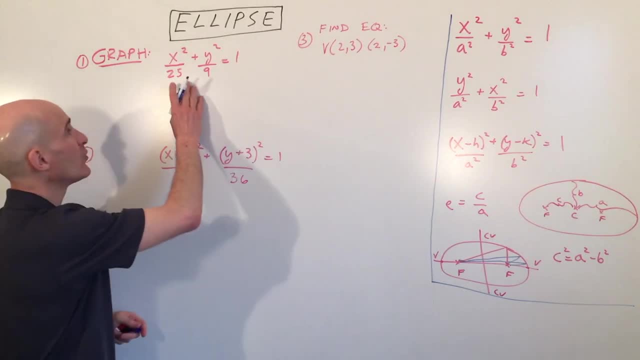 bit more about it as we we do it. So this first example we have: x squared over 25 plus y squared over 9 equals 1.. Okay, so if we go to graph this, we can see that 25 equals a squared. Okay, so what? 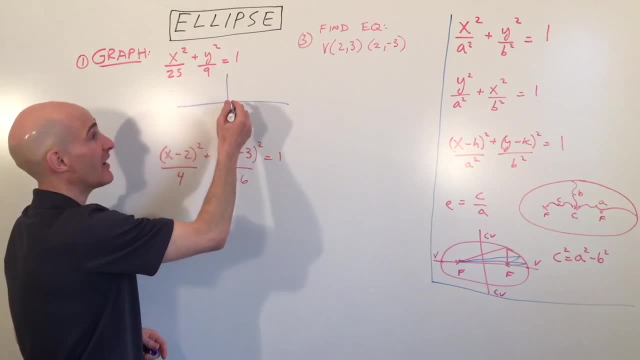 I'm going to do is in the x direction. I'm going to go right 5 and left 5.. I'm just taking the okay. so those are our vertices. and then if we take the square root of nine, we get three and negative three, and it's easy to remember because it's underneath the y. so it's going to go in the 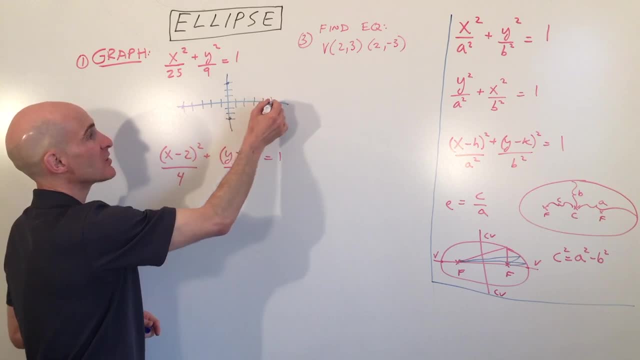 y direction, the vertical direction: up three, down three. so at this point we have a pretty good graph. you just draw an oval or an ellipse, okay, through those points. but the only thing we're missing is how to find the focal points, the foci, and the way you do that is use this formula here: 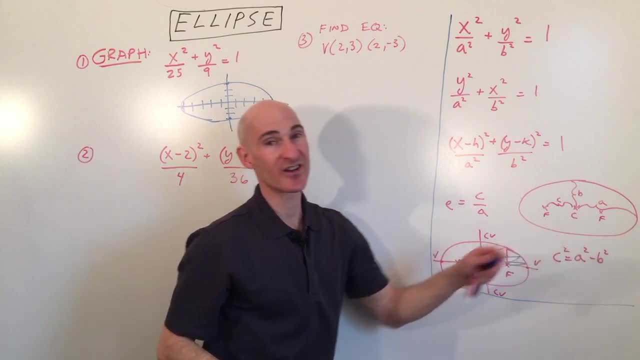 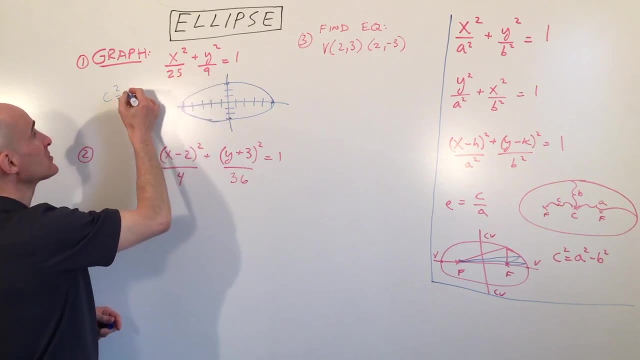 it's: c squared equals a squared, minus b squared. okay, so in this problem, here it's going to be: c squared equals a squared, that's the larger of these two denominators. it's 25 minus 9, which equals 16, and if we take the square root, we get plus or minus 4, so the foci are always going to. 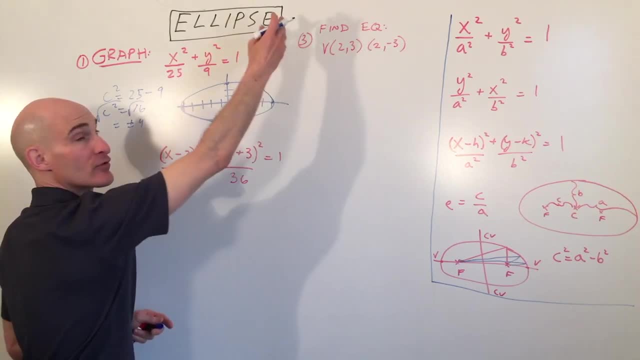 be along the longer axis, the major axis. if it was longer in the vertical direction we'd be going up and down. so i'm just going to go right four and left four. those are the two foci right there. so if we take the square root of nine, we get plus or minus four. so the foci are always going to be. 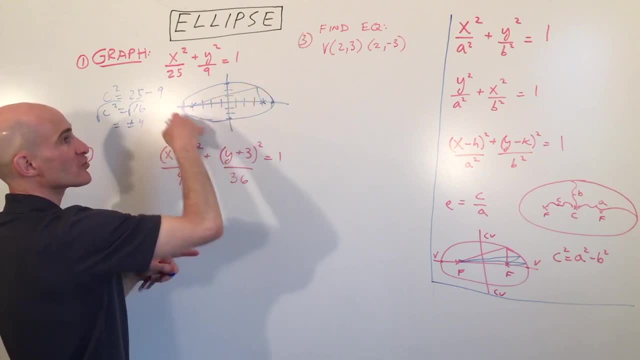 if we were to tie our string, we would hold it down there and that's what would trace out the ellipse. okay, let's do another example, this one you can see. the center is where it's at positive, two, negative, three, right, okay, so if we graph this one, 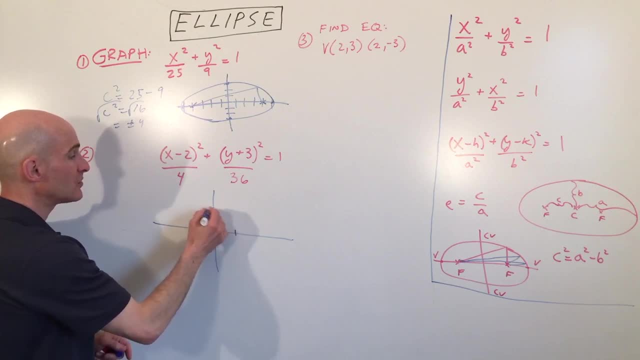 let's locate the center right. two up three, okay, like that, and i think i'm gonna have to give myself a little bit more room for this one, so i'm just going to write: draw it a little bit lower, okay. so let's go down here. so we've got right. two: 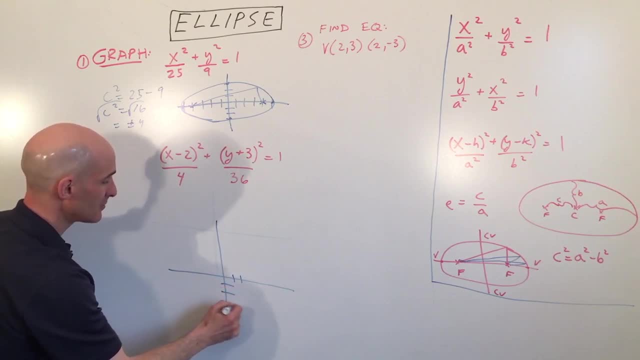 uh, plus three is down three, okay. so there's your center right there, and then what we're going to do is we're going to go two in the x direction, so the square root of four is two. so i'm going to go two to the right of the center point, so right two and left two, okay, and i'm going to go in the y. 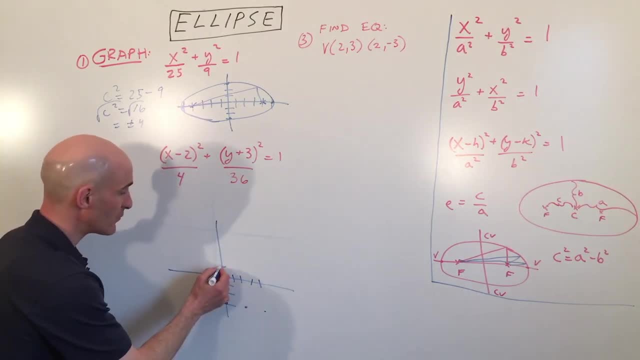 direction the square root of 36. so up six and down six. so that's four, five, six. okay, right there. and then down six, one, two, three, four, five, six. so right about there, okay, oops, i went a little bit too far right there, okay, so if you graph this, okay. 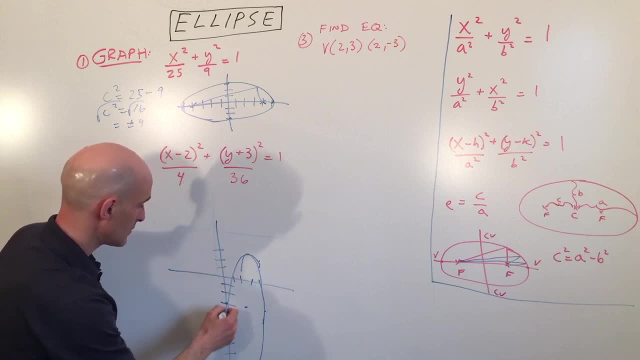 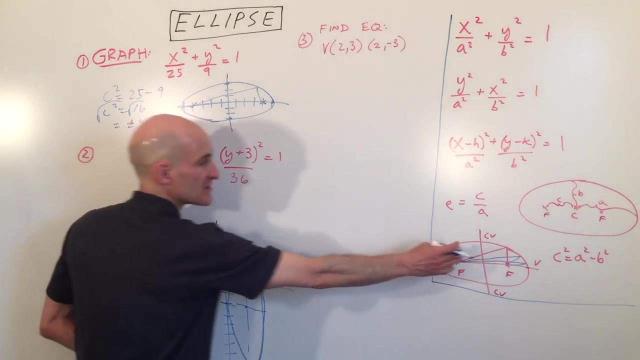 okay, your ellipse is going to look something like that. okay, so this is the major axis, this is the minor axis, this is the center point. the only thing we have left to do is to find the foci, and we're going to use the same formula: c squared equals a squared minus b squared. 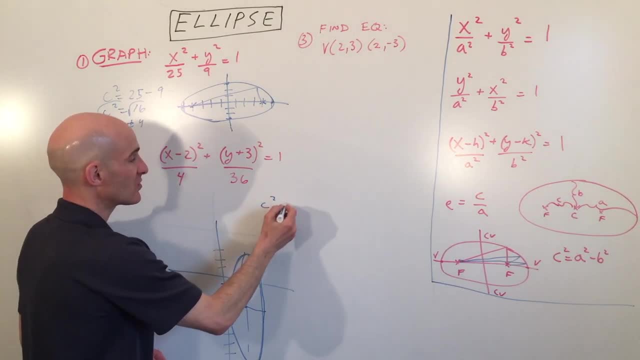 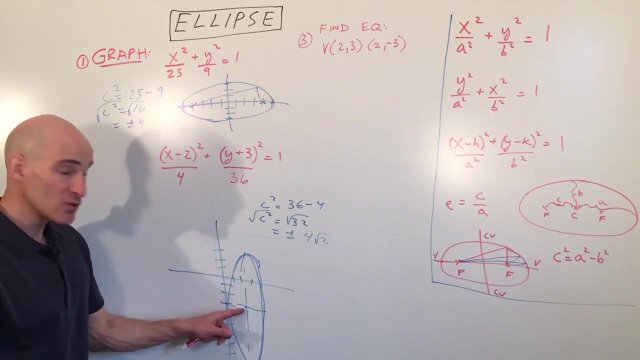 remember, a squared is the larger of these two denominators. so we have c: squared equals 36 minus 4, which is 32, and if we take the square root we get plus or minus. square root of 32 is 4, root 2, because 16 times 2 is 32. but what we want to do is we want to go from the center point, which 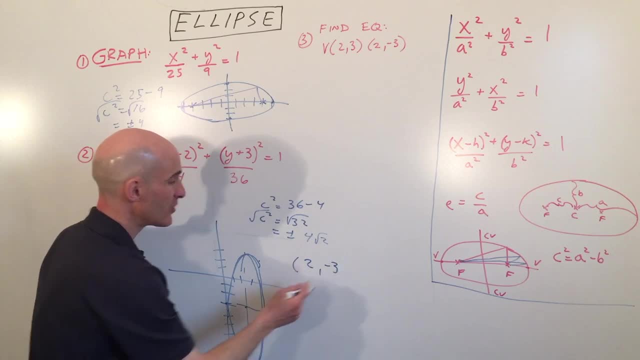 is 2 negative 3, but we're adding 4 root 2 and subtracting 4 root 2 from the y coordinate, since we're going in a vertical direction. so this is going to be plus or minus 4 root 2. those are the. 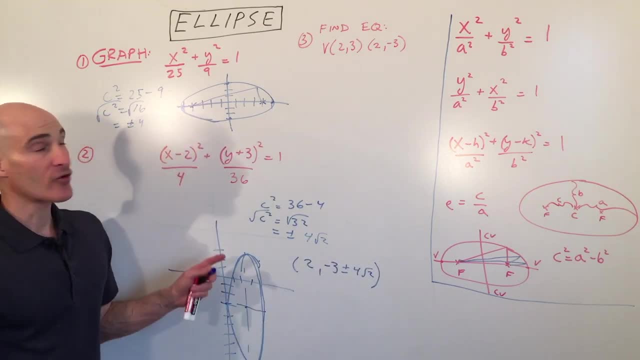 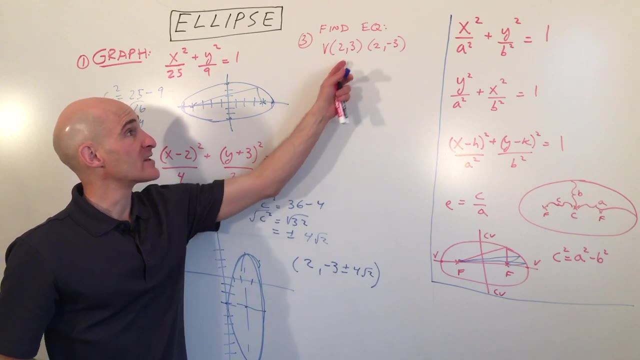 coordinates of the foci. okay, all right. so that's a little bit about graphing. now, how about working backwards, where they give you some information and you have to come up with your own equation? well, i still recommend drawing a sketch. that'll really help you to get all the pieces together- the a, b and c. so let's go. 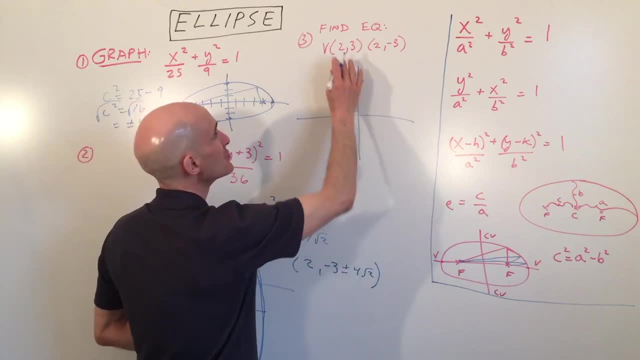 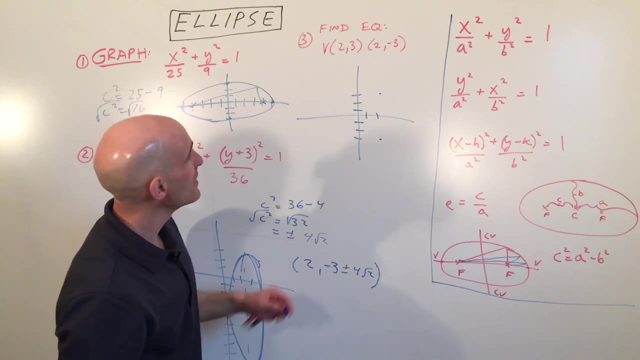 ahead and graph this. okay, so the vertices they're telling us are at 2, 3 and at 2 negative 3. okay, so you're with me so far. so those are the vertices and we're going to need a little bit more information here. okay, i just made this problem up off the cuff here, but let's just say that the foci, okay, are at: 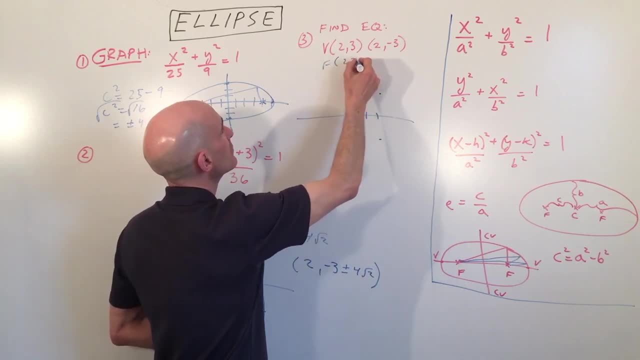 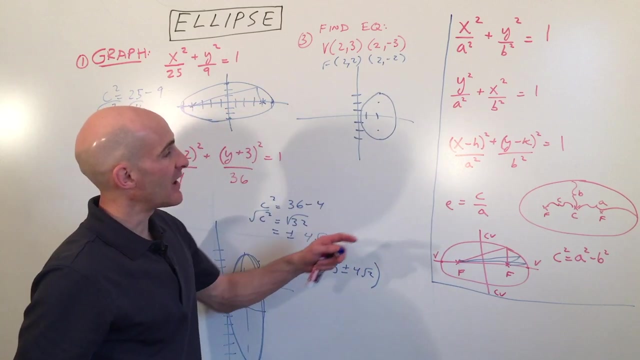 2- 2 and at 2 negative 2. okay, so they're going to be right here and right here. okay, so we can see that our ellipse is going to look something like this, and we don't know how wide it is yet, but we're going to figure that out using this formula: here: c squared equals a squared minus b squared.